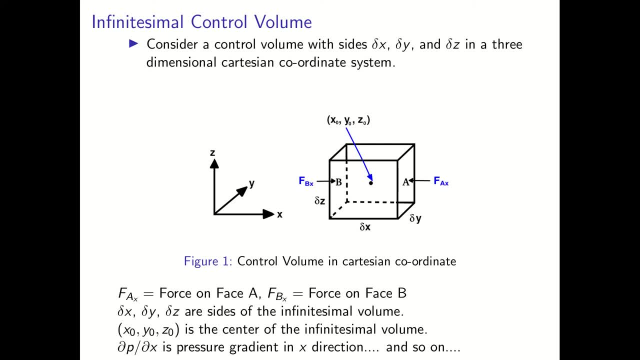 delta as the gradient. So in an infinitesimally small control volume you will have the gradients of pressure in all the 3 dimensions: x, y and z. Let's say, the gradient of pressure in x direction is delta x. Similarly, you will have the gradient of pressure in y and z direction. 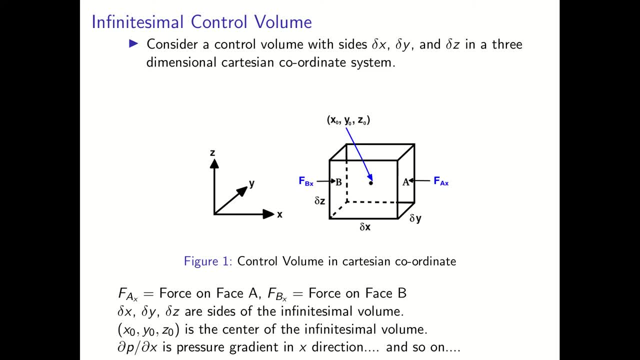 as del p by del y and del p by del z. let's say that the center of this cube, that infinitesimal cube, is x0, y0 and z0, and our focus is to formally calculate the resultant force F due to the three gradients of pressure in the three directions, three dimensions. 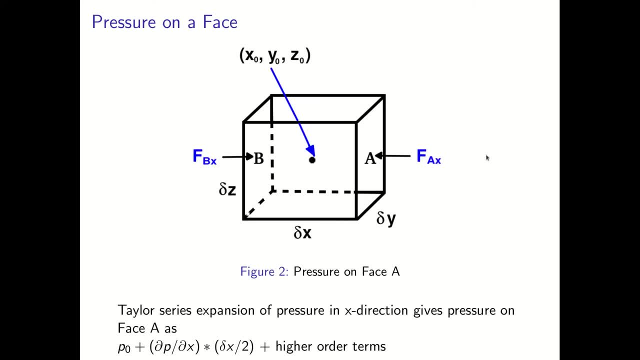 ok, let's say, if you want to calculate the resultant force, we have to calculate the forces due to pressure gradient at various surfaces. so we'll start with the one dimension in x dimension, and let's say that the force acting on the face A of this cube 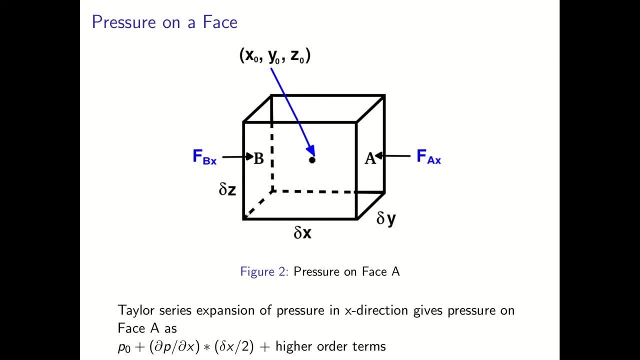 is x0 minus E is Fax and the force acting on face B is Fbx. Now, since the distance between the center of the cube and the face A is delta x by 2 and the similar distance is between the surface B and the center, we can multiply this distance with the gradient of pressure, so that the resultant pressure at 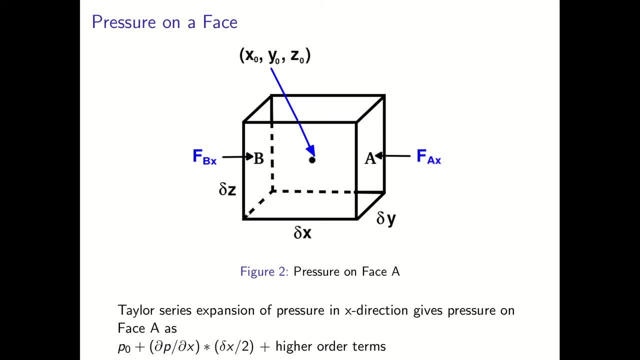 surface A is P0 plus del P by del x and multiplied by distance, so delta x by 2 and we will have the higher order terms also depending on the gradient of gradient itself and so on. But in this lecture we will basically drop these higher order terms and we will focus. 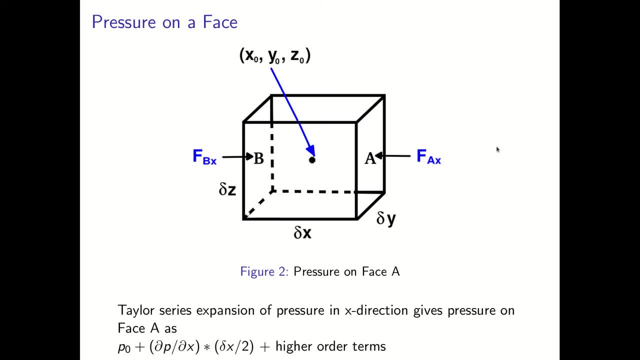 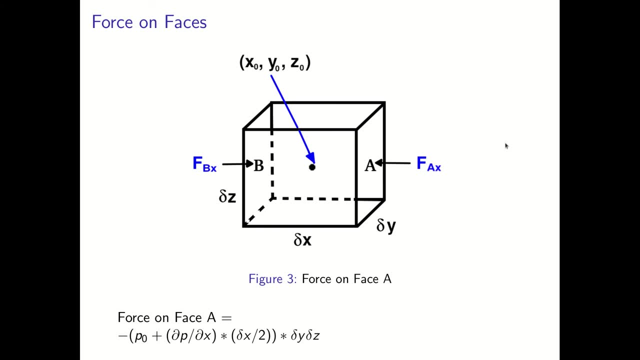 only on the first term of the Taylor series. okay, So similarly you will have the pressure at the other faces also. So given the pressure on the face F A to be P0 plus delta P by del P by del x into delta x by 2, we want to calculate the force. So force. 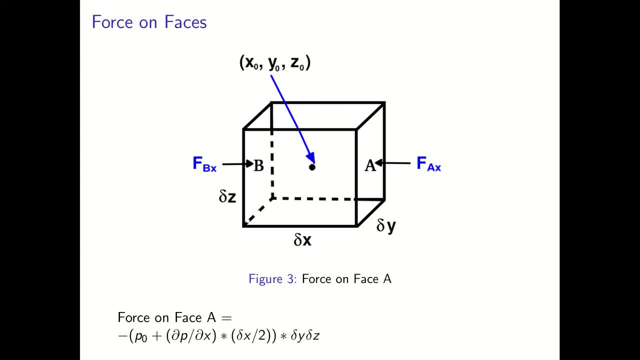 is pressure is basically force per unit area. So the force itself is pressure into area, and the area of the face A is delta y into delta z. So you multiply this by delta P, by the area of the face P, and see, we simply substitute the force as resolution. 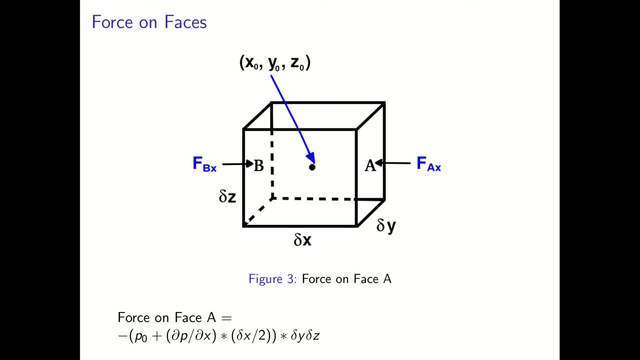 of the phase A and the area of the face where we want to report it is appningen. So here the area of the face A will be force hauled from that x-axis and you can see about. the area along the face S will be equal-squared act with the area. começa to oppress this. 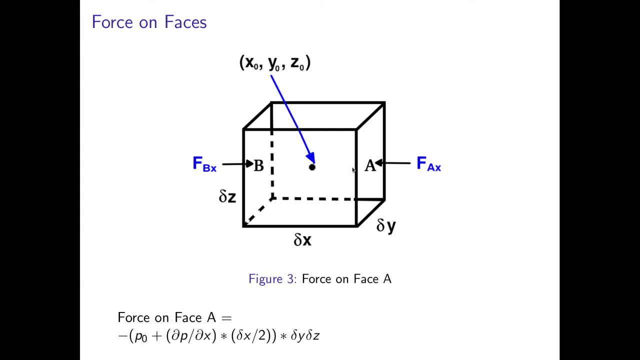 part of the face and for theةx direction will be equal-squared act and there will also be force hauled along the face S all right, So that's when we also make some calculations. So this means when we理itialize this surfaceדm, there will be some pressure which will be running. 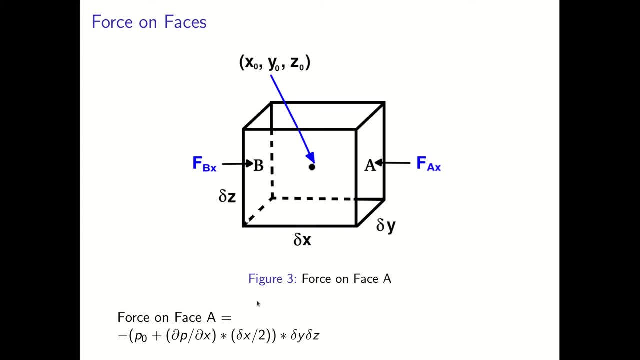 along the face aN and theговιw would also be a slope at the face A. So we will simulate as the surface of this surface where if that side of the face is classed, then at the opposite side, the. So this is the final expression that we get for force at phase A and similarly we can calculate: 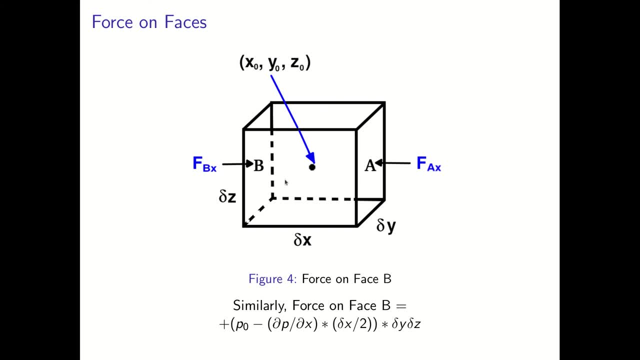 the force at phase B, Note that there will be two differences. one that will subtract delta x by 2 from x0. So you will have minus of delta x by 2 multiplied with the pressure gradient and the force is in the direction of pressure gradient. So FBx is in the direction of the. 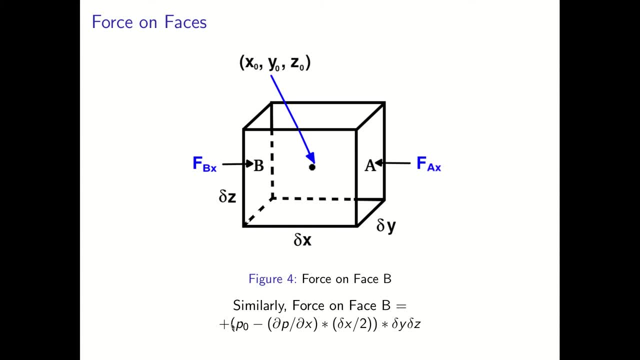 pressure gradient in the x direction. So we will be using a positive sign here. So the force on phase B will be P0 minus delta. P by delta x into del P by del and del P by del x into delta x by 2 and multiplied with the area. So delta y into delta z. 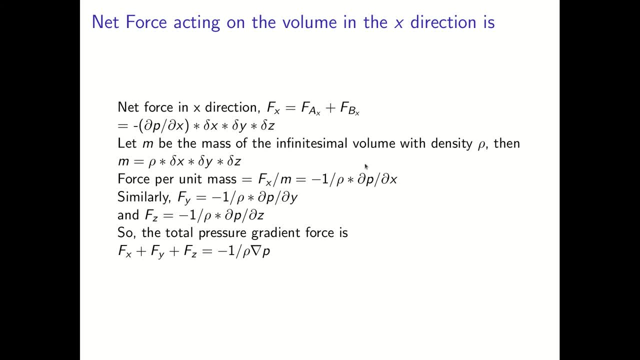 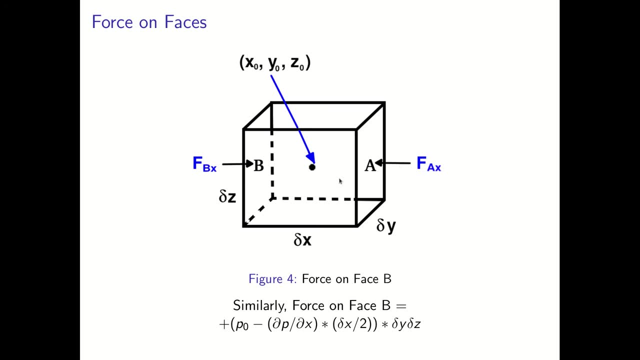 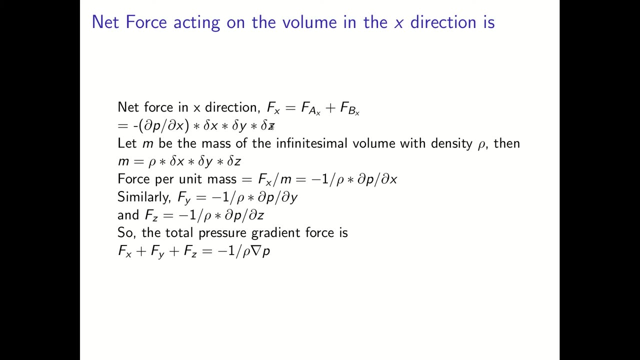 Now the net force itself will be the summation of two forces. So the net force in the x direction will be FA plus FB, So vector sum, And if we basically take these two terms and add them together, what we are left with is minus del P by del x. So if you look at the expression for the force for B,